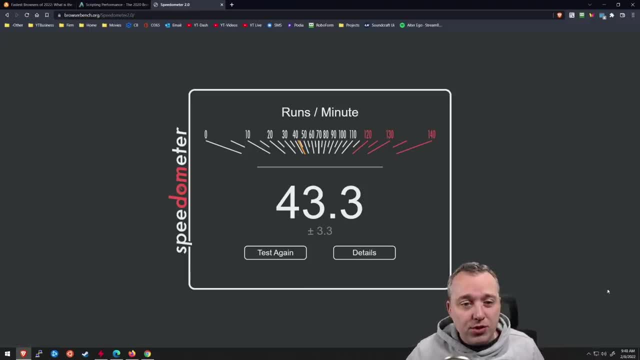 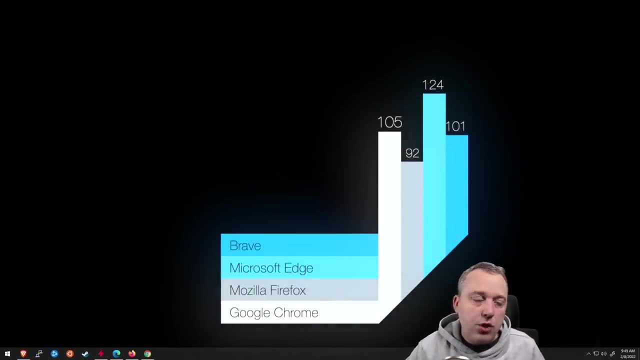 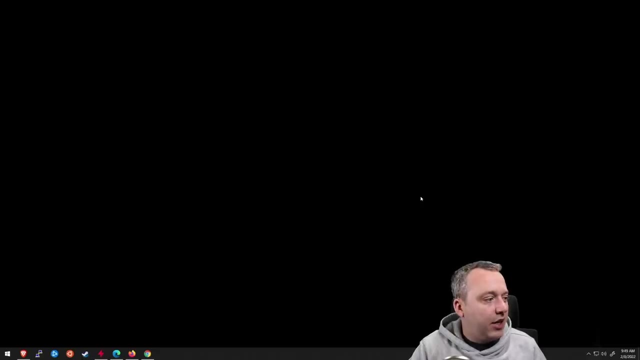 was right for you at the end here. Now, before we get started here, this is what Avast shows. This is the entire speedometer range. Then I went and installed Microsoft Edge, Firefox, Chrome, and then I may have tossed in another couple in here. I did it in both Windows and 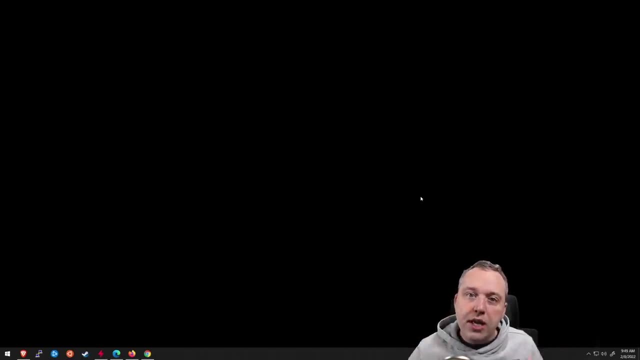 Linux. So let's get to that, so you understand what's happening with each one of these and which one is the fastest browser. But before we do that, I just want to say I don't like each one of these browsers for different reasons, So I'll lay those out real fast here and we'll talk again at the end. 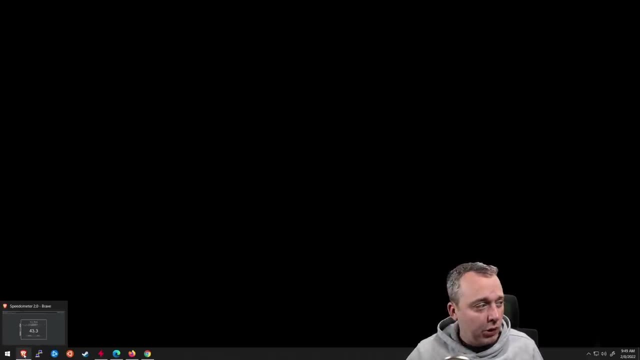 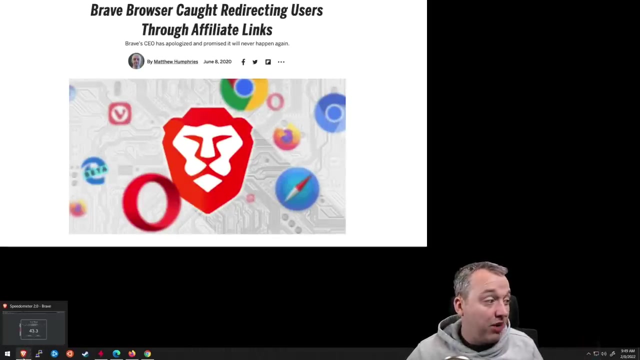 about that. Brave I don't like for its involvement with a lot of crypto type stuff and some of the dodgy history with search redirection to get affiliate links and some other things. Even though I do use Brave as my primary browser, it does have some bad things going for it. Microsoft Edge is. 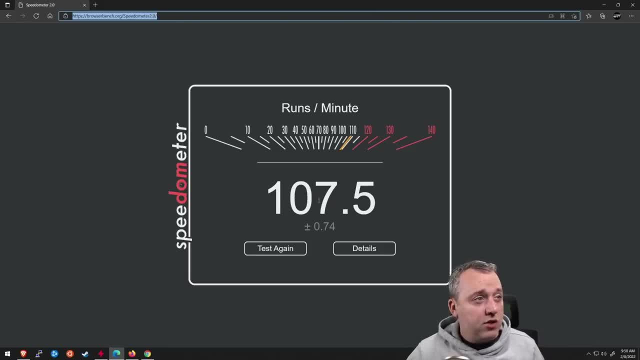 the next one, which I showed right here at 107.. This is often known as the fastest browser on the web, but that's actually not true anymore. Back in 2018, this was the case when they first released Chromium- No longer. You'll see here in a minute. 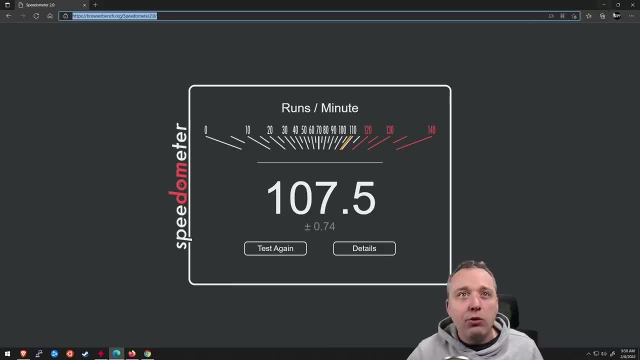 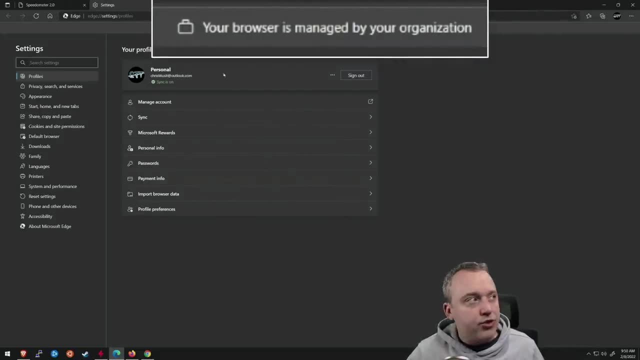 But the big thing about Edge is it integrates really tightly with the operating system. So if you ever do any tweaks, disable any telemetry, do anything, you're going to get this browsers managed by your organization And then it kind of locks down most of the things in Edge And it 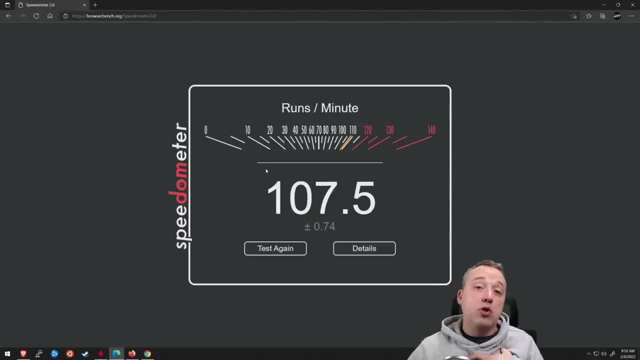 kind of is a terrible browser because of that, because I do so many modifications. However, if you just leave everything stock and you just leave all the bloatware that comes with Windows on your system, that's there. However, I wanted to see what this performance would be like. 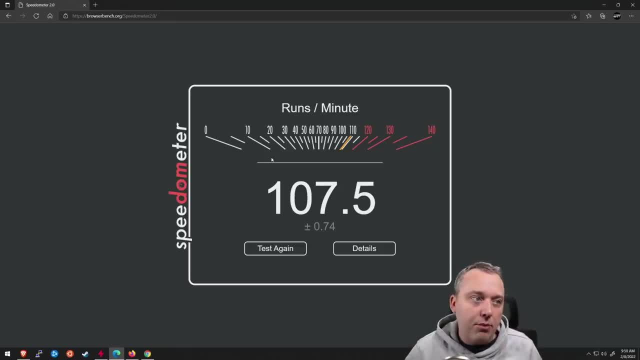 I'm not sure if it's going to be the same as it is in Linux, where it doesn't have that integration into the operating system which I'll show here in a second, Because I was really curious to see how much of a leg up Edge gets because of Microsoft Windows, which is something. 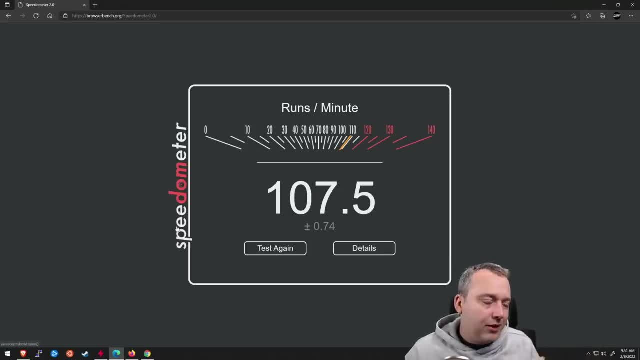 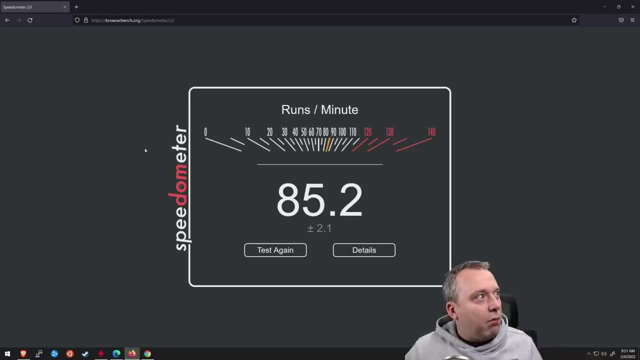 I was like, oh, maybe that would be a whole video in itself. Spoiler: not as much as you think. Firefox- you know Firefox's performance has always been a little bit lacking, but I love it because it's pretty much the only independent browser. Everything else I'm showing: 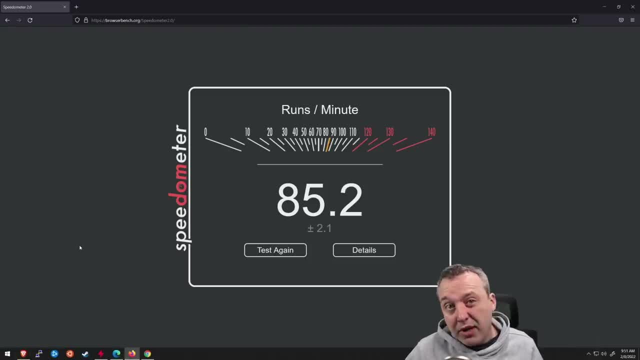 Edge and Brave. they're all Chromium based, So they're basically controlled by Google, or not controlled, but based on Google's code or the Chromium code. But yes, so I always recommend people use Firefox, even though I don't. it's not my cup of tea, so to speak. I don't really have 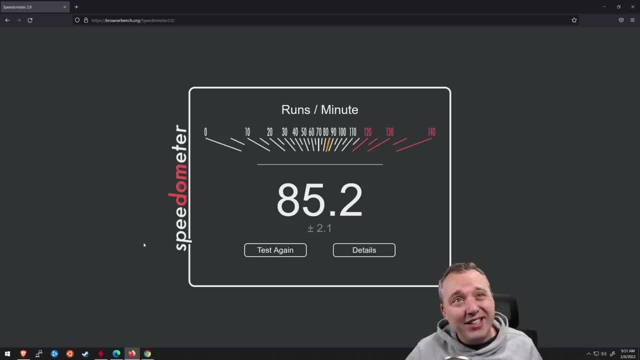 anything too negative to say from it. Otherwise, I don't really like its ecosystem that much. It feels a little bit foreign to me because I've always used a Chromium based browser. but I don't want to discourage anybody from using Firefox because it is pretty much the only competition. 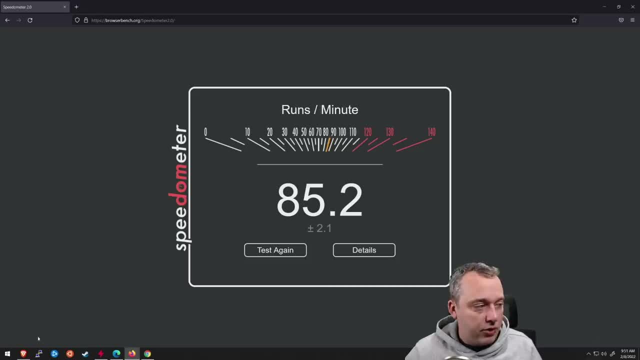 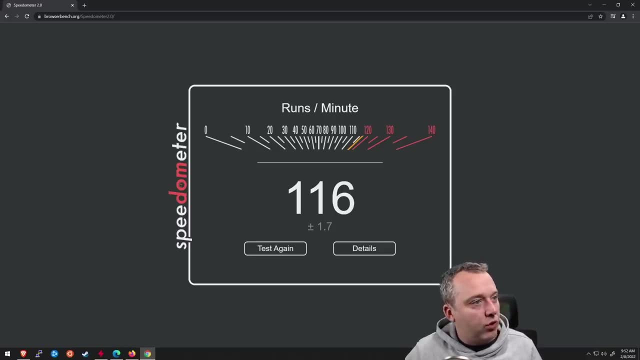 to a Google Chromium based browser, as these other ones I'm showing are all Chromium based. And then finally, Chrome, And you'll notice it has the highest score in 2022, and it's pretty darn responsive. But this is all just using speedometer, And one of the flaws to 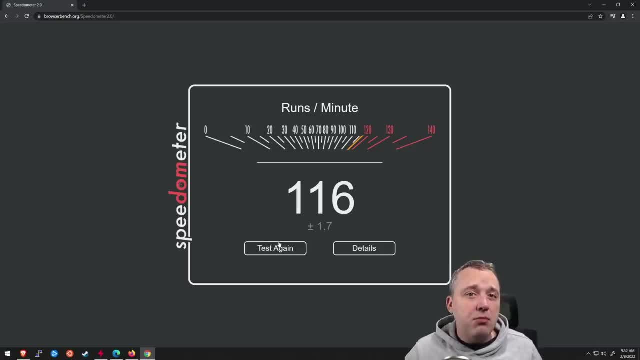 just using this test is: every website's a little different. Some browsers will be faster on other websites and some browsers will be optimized for certain websites. So if you want to skew these to whatever you want to show you, you can. But this was the final scores in Windows. 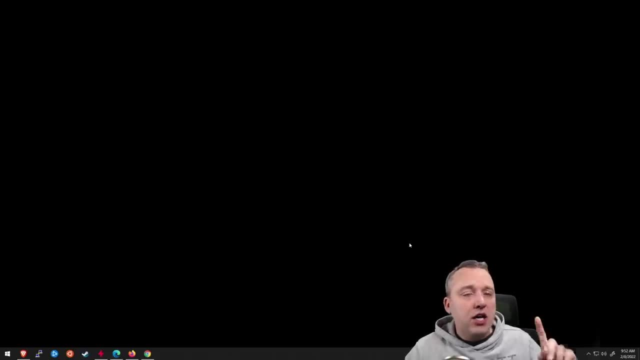 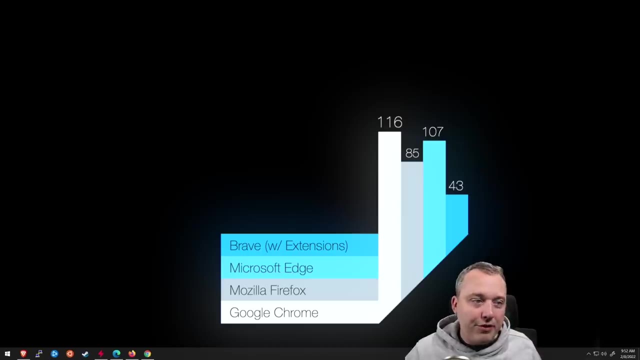 and we're going to move to Linux next. Let me just minimize this. Here you go. That is what we got for Windows, And now let's move into the Linux realm things- and flip over into it. So here is the Linux desktop. I went ahead and 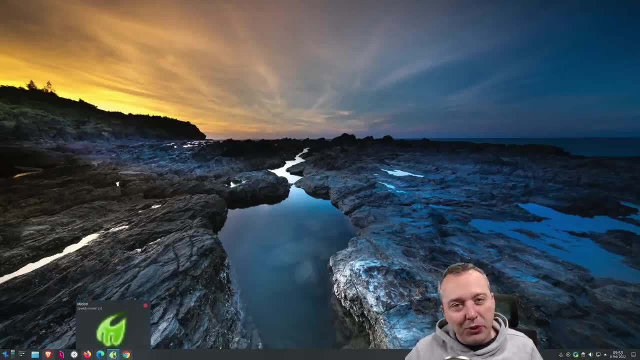 lost another one in here called Midori. It's like this bare bones browser And I was like: what does it do on a speed test? I was expecting it to be the top one Again. spoiler- no, it's not. 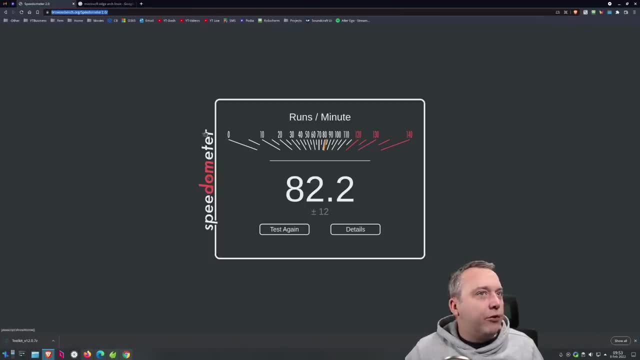 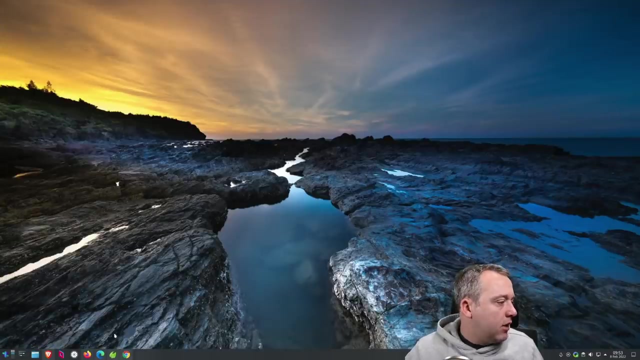 All right, So we'll start with old Brave over here, loaded down with all my extensions and all my bloat- double the score compared to Windows. Not that shocking, because obviously Linux is going to be a lot more lightweight- not so much running in the memory, And then 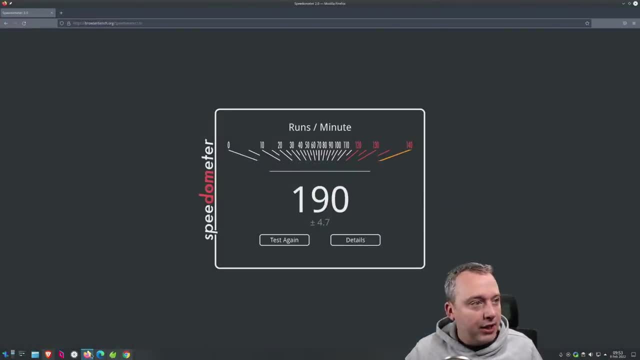 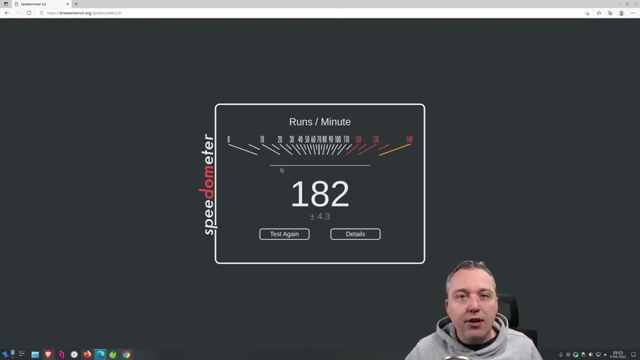 Firefox 190, considerably better, almost double again from the Windows counterpart Edge, again really good. Surprisingly this one came in a little bit lower than what we saw with Firefox. That's the first time I've ever seen Edge come behind Firefox, but it's kind of interesting. 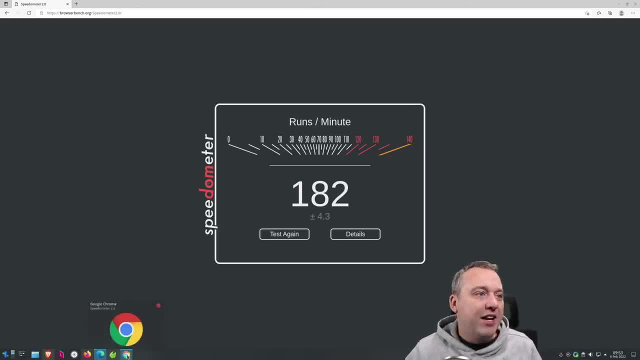 You'd be thinking it would be double, much like the others, but you'd be wrong. And then finally, Chrome at a whopping 234.. That's nuts. And then just to kind of throw things in to Midori, which is a bare bones, I think it's. 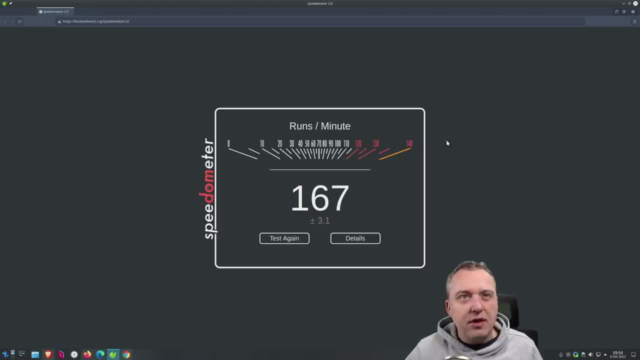 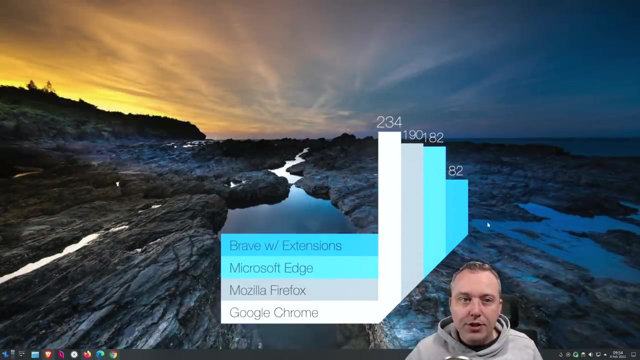 actually Chromium based browser with no extensions. 167, about pretty underperforming. I really expected this to be the best and it's not So that was kind of interesting going through the speedometer test, The final results on your screen right here. Chrome whopping the competition. 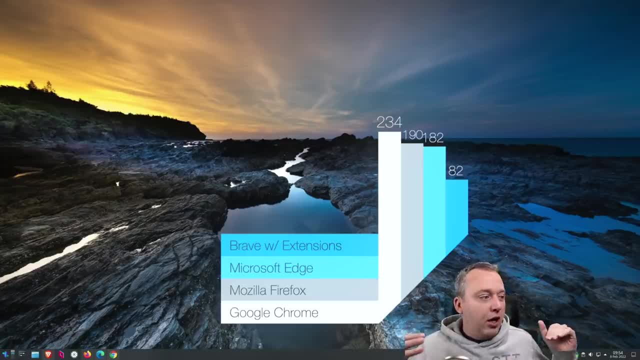 by that metric, But I kind of want to show these Now. I thought I gave every advantage to most of the other browsers on here. I gave every advantage to most of the other browsers on here. I gave every advantage to most of the other browsers on here. 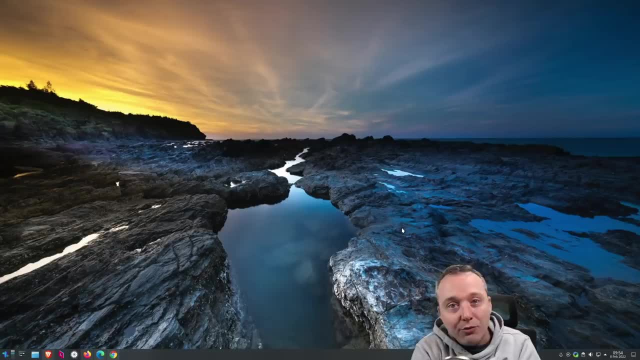 Because I honestly don't want people to use Chrome because it's kind of tied in with Google. But that's the downside to Chrome is you're in the Google ecosystem. but it's also the upside: If you're really into Google ecosystem and you want to stay there by all means, you can use. 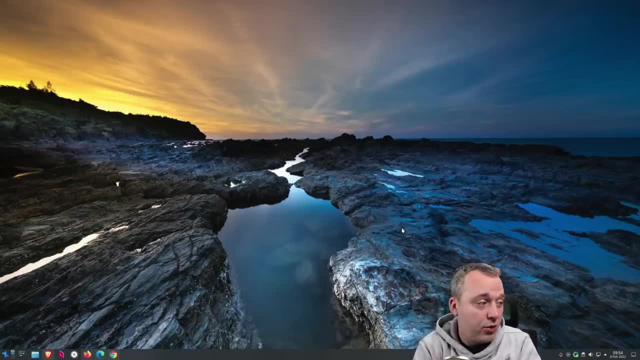 Chrome because it is fast And I think it is the fastest browser based on every test I've run in 2022.. They've done some good optimizations to it. A couple other notables in here that I left off was Vivaldi. I need to check them out again. 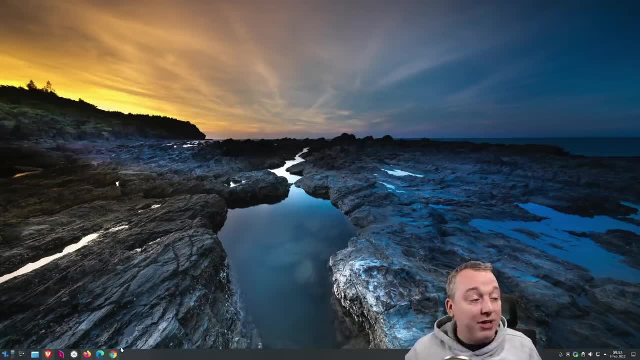 Originally used to use Vivaldi in a switch to Brave, mainly because of performance based issues. It was really kind of getting laggy. I had a bad update And I think since they've fixed all that, I still like Vivaldi. One that some actual tests show is Opera. Don't use Opera. The company behind 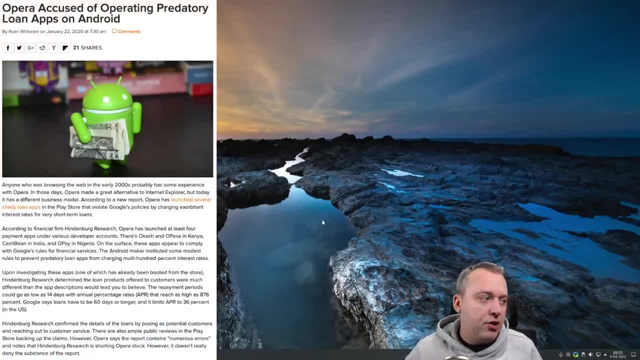 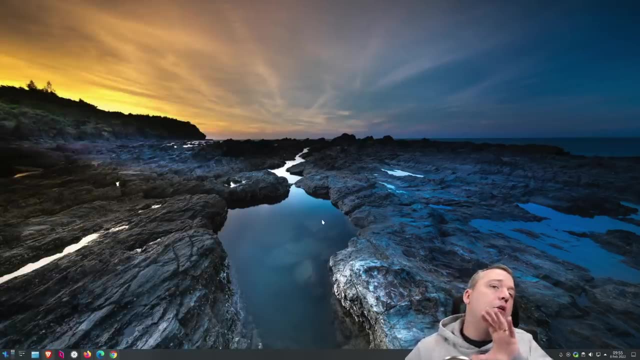 it has done some very shady practices, especially in the mobile space where they'd sign people up with loans, And it was just a really shady company. The founder of Opera actually moved on to create Vivaldi, Or one of the founders, I should say, moved on to create Vivaldi. So if you like the way Opera